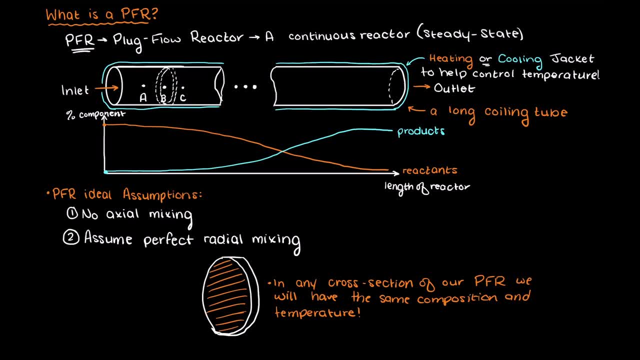 section. Therefore, because of these two assumptions and with how the PFR is set up, that we track the changes in our fluid's composition as a function of distance through the PFR rather than time, like we did with our other reactors, like the batch, semibatch and CSTR. 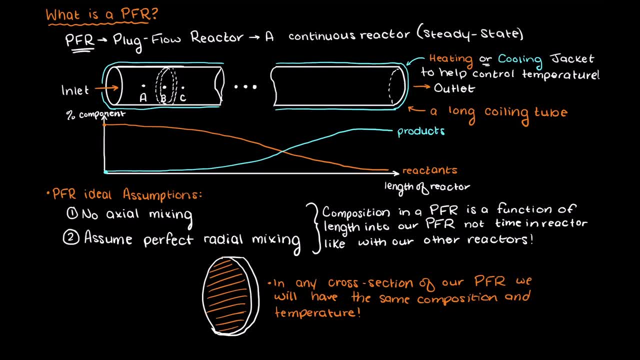 So if we were operating our PFR here at steady state, then 1 meter into our reactor should always in theory give the same composition, whether we test that composition now or in an hour from now. So lastly, because our plug flow reactor is a steady state reactor, that means that 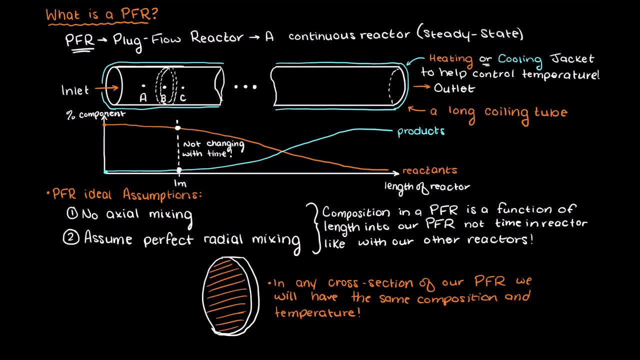 when operating, we continuously would be feeding it reactants and removing products at the same time, The idea here being that new reactants enter our tank, stay reacting for a certain amount of time, called our residence time, and then leave the reactor once the reactants 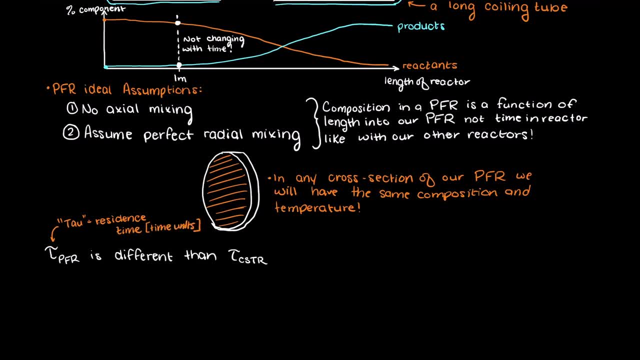 have all become products. I should note that when we are talking about the residence time of a PFR, it is slightly different than a CSTR, So if we were operating a PFR here at steady state, then we would be feeding it reactants. 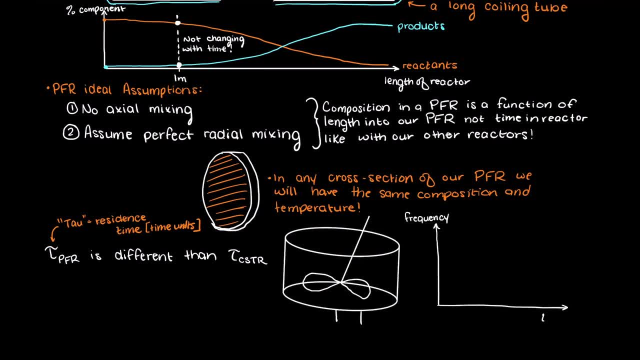 and removing products at the same time. That would be the same as when we were operating a PFR In a CSTR. the residence time is a distribution based on statistics and that is why it looks like a bell curve. It is based on the average time, an average particle. 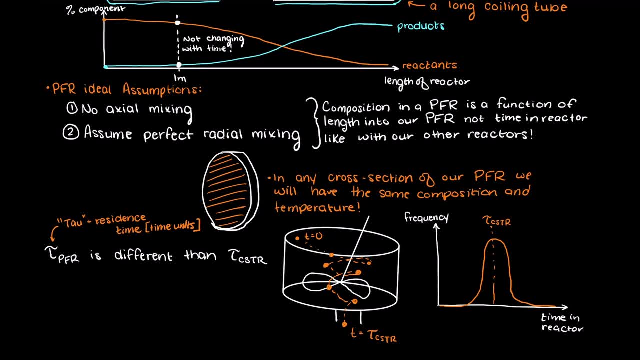 spends in the CSTR, Whereas in a PFR we just have a single residence time, as we are assuming that the fluid is continually and always moving forward at a constant rate. This is why we call it a plug flow reactor. You can imagine this little plug shape here acting as 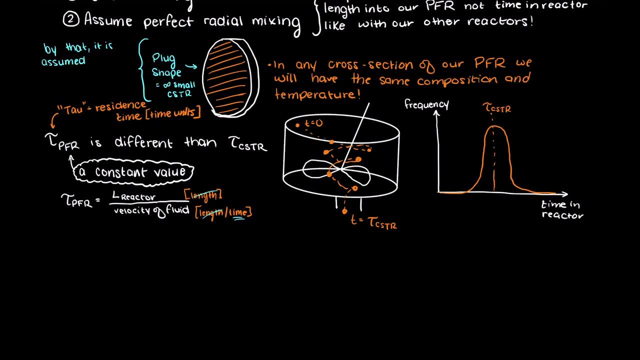 an infinitesimally small CSTR, and by stringing our infinite amount of CSTRs together we get a plug flow reactor. Some advantages to PFRs are that they are great for gas phase and liquid phase reactions. Additionally, we can experience fast reaction times in a plug flow. 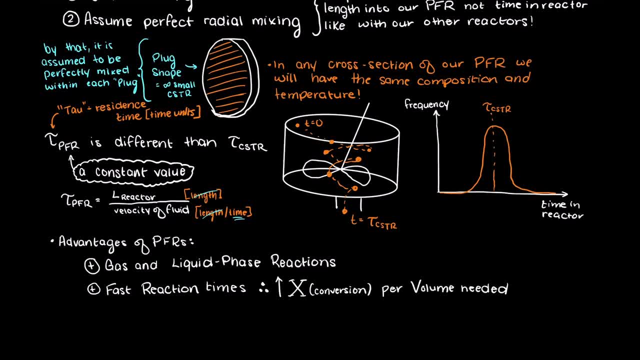 reactor and therefore we have high levels of conversion for the volume needed, unlike CSTRs, which we talked about in the last video. Operating continuously is great for industrial scale up of a reactor. This is why we call it a plug flow reactor. This is why we call it a plug flow reactor. 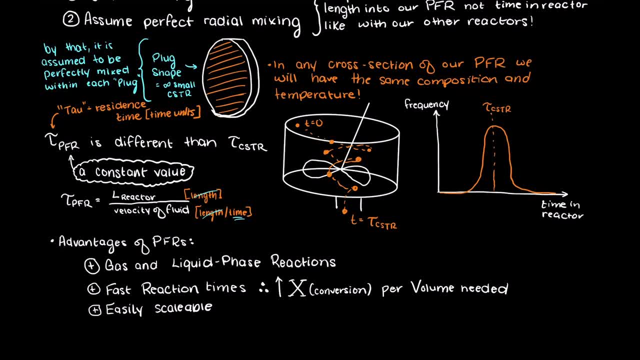 We can also achieve higher temperatures in PFRs, which is something necessary for some reactions. Another benefit is that we have lower labor costs, as the reactor will mostly be running itself as it is in a steady state. However, because it is just a long tube, sometimes cleaning the PFRs. 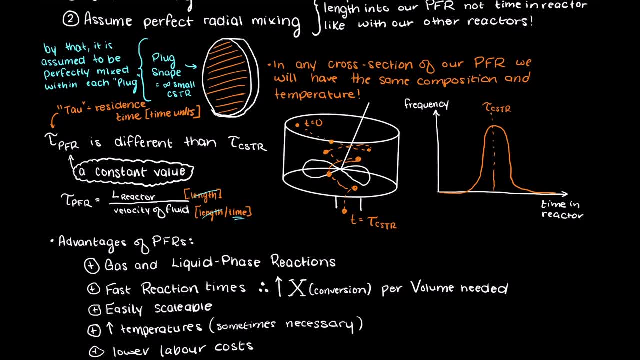 can be a challenge to make sure that it is properly sanitized upon shutdown. Also, shutdown can sometimes be expensive, depending on the type of reactor you are working in. This is why we call it a plug flow reactor. This is why we call it a plug flow reactor. This is why we call it a plug flow. 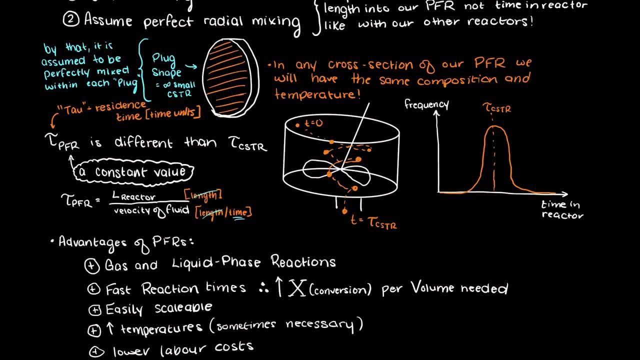 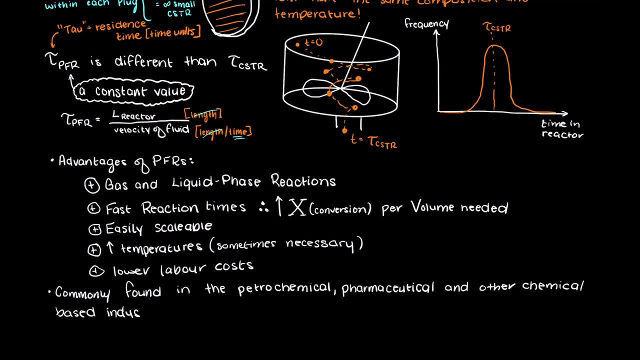 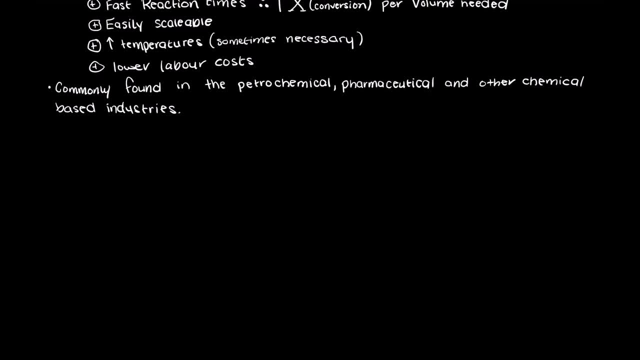 pharmaceutical and several other chemical based industries. Now that we have an understanding of what a plug flow reactor is, what they look like and how they work, we can talk more about the general mole-balance around a PFR. We introduced the mole balance in a previous video. 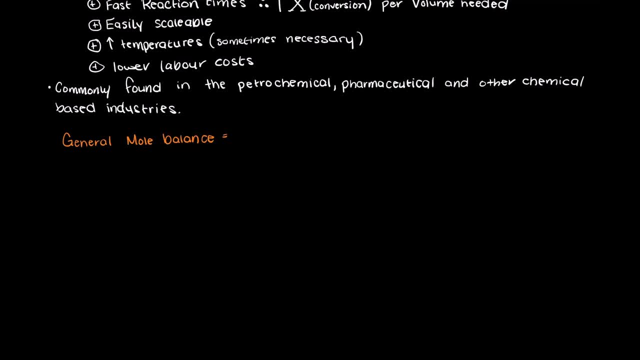 and I will leave a link for you in the description below, below, if you'd like to check out the video. So I've just written the general mole balance here and we can eliminate any terms that we don't need. So we are studying one constant area of our plug flow reactor over time. 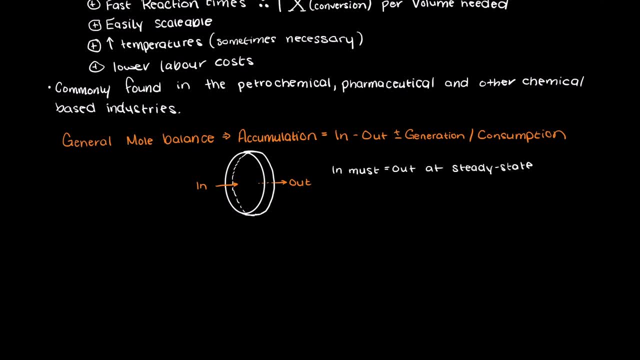 So just remember that. we mentioned earlier that the inlet and the outlet to the reactor must always be equal, otherwise we would not have a steady state. So this means that our accumulation term will be zero, and this will always be the case for a steady state system. 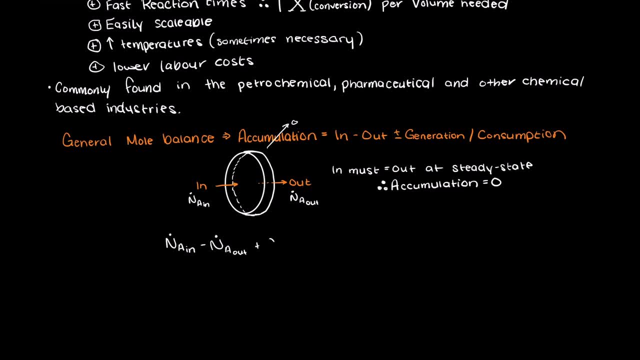 So we just have the moles of component A coming into our system, minus the moles of component A leaving our system, plus the amount of moles of A generated within our reactor, minus the amount of moles consumed within the reactor. So this term here could be the generation of A or the consumption of A, or both depending. 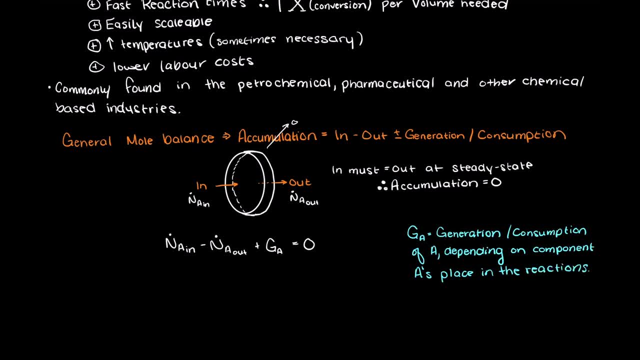 on what part component A plays in the reaction. Just note that GA here stands for the generation or consumption of component A. therefore, it is equal to the rate of formation in the terms of generation or rate of accumulation. We would talk more about this in coming videos, though.